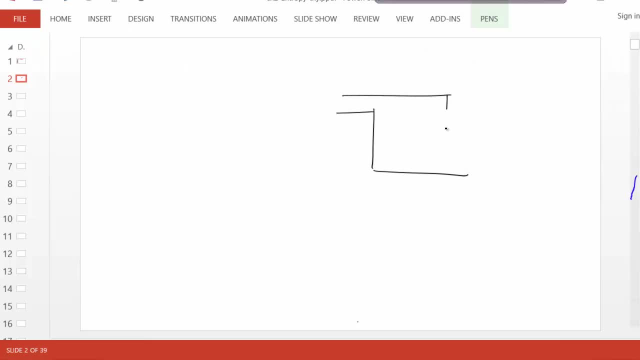 Well, I'll draw a simple system, but you can use your imagination to make it more complicated. So let's say we have an inlet state I, an exit state E of an open generic system. And let's say we have some shaft work transfer. Let's say a pedal wheel is turning. 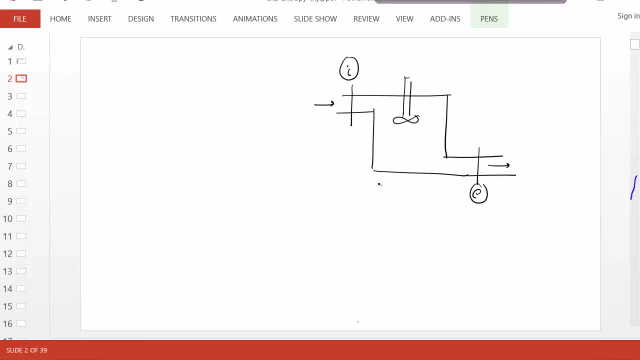 And also let's say that heat is being transferred here Into the system. Let's do a system boundary, OK. so we want to develop the entropy balance equation for this system. Simple thing first: We understand: as mass goes in, it carries entropy with it. 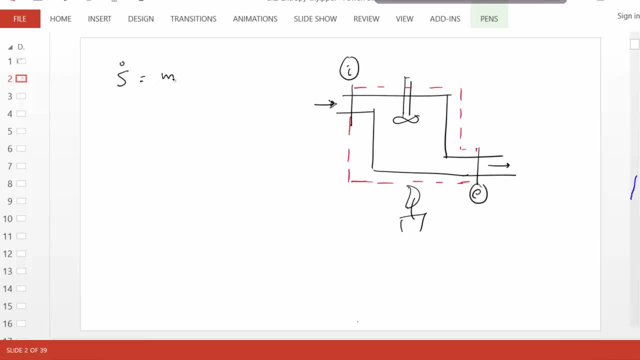 So entropy transport S dot would be simply just M dot S. If you recall that flow, energy transport is given by equations such as this, These are called transport equations. So as mass goes in, it will carry entropy in. As mass comes out, it will transport entropy out. 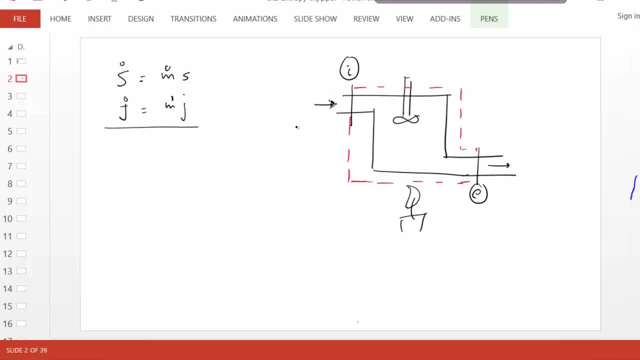 So we have entropy going in at the inlet location would be M dot times S, I, M dot I times S I and here M dot E times S? E. Well, to understand what, What will happen because of the work and heat transfer to entropy. 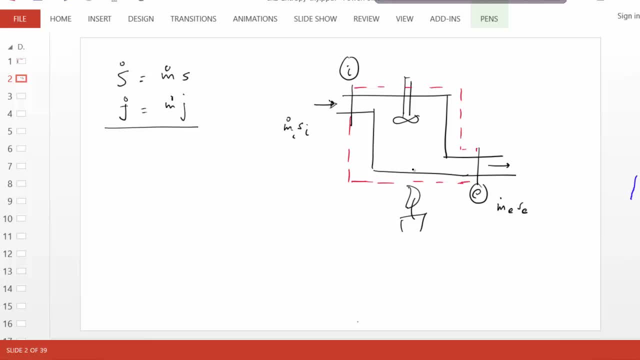 We need to go back to the definition of entropy. If you recall what entropy is, Entropy is given for a big system, K times ln, omega, Where omega is the number of ways in which the internal energy of a system can be distributed amongst its molecules. 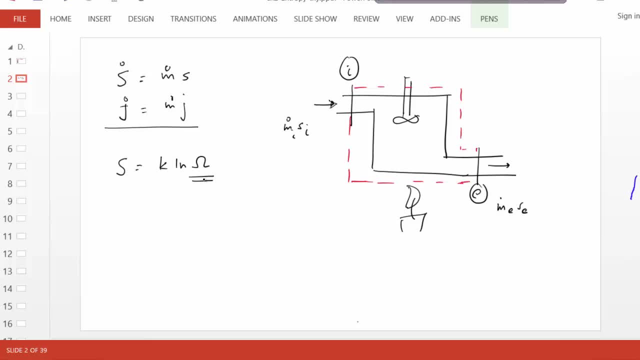 So it sounds like a very abstruse Abstract concept. So let's try to simplify the idea and see if we can get an intuitive understanding of what happens. So essentially, Entropy is a measure of in how many ways energy can be stored. 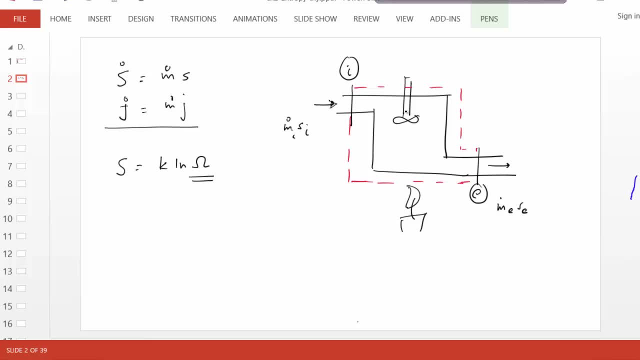 So it's a kind of a measure of the disorganization inside the system. So let's say, and we also recall from our fundamental understanding, that The energy is the internal energy is distributed amongst its molecules, molecule being the smallest unit of a system. 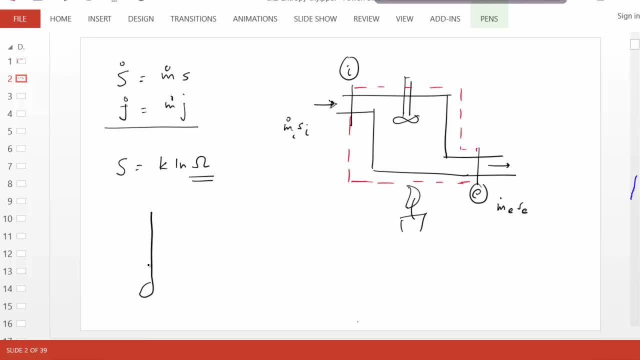 So each molecule in our model, if you recall, will have a letter of energy levels, And we also know if the temperature of a system is higher. Of course the molecule will have more energy, but it will also have more levels of energy. 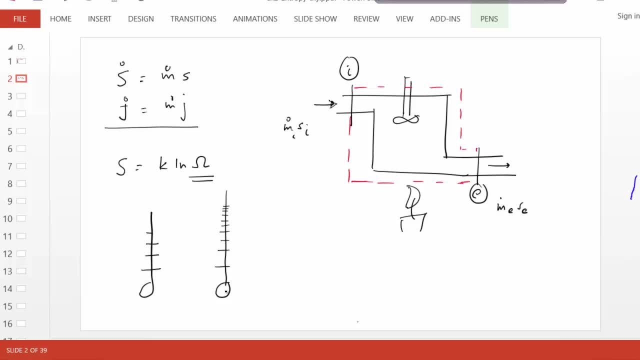 And that's also intuitively understandable. If the temperature is higher, more doors are open to a molecule. If temperature is really really high, even electrons can start jumping from one or between other, opening up even more ways to store energy. Of course, we know that as temperature increases, the temperature being a measure of the kinetic energy of the molecules, is kinetic energy increases. 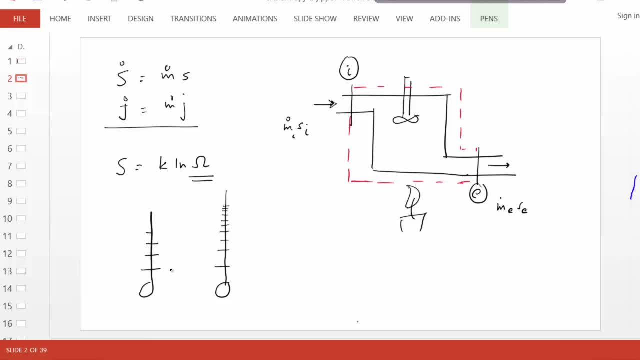 But it is. it is nice to have a picture in your mind that the higher the temperature- let's say, this is a system at 1000 Kelvin And this is a system at 500 Kelvin, So here maybe the molecules can be stored. 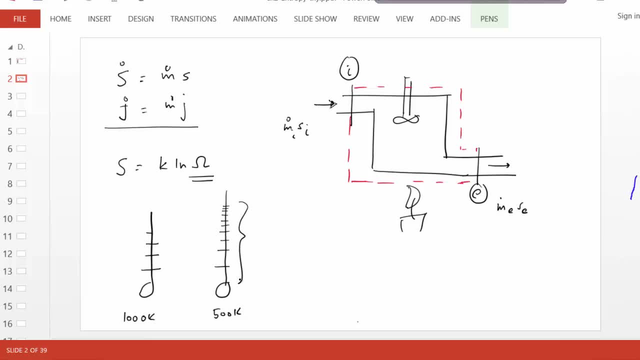 Let's say I'm just taking an arbitrary number, I'm sorry, this would be 1000 Kelvin And this is our 500 Kelvin case. Just suppose here the energy can be stored in 10 ways, Then here probably, the energy can be stored in 50 ways. 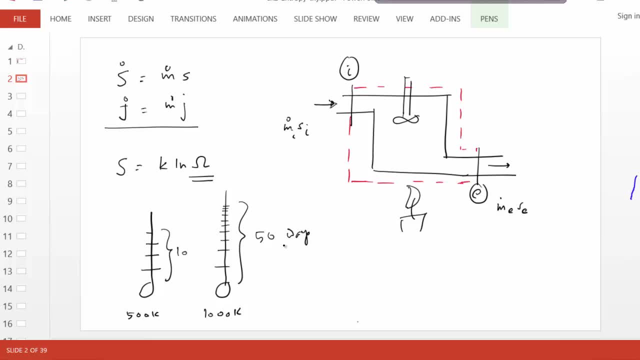 50 different levels. Okay, so we'll keep this model in our mind, But let's try to understand what happens when heat crosses the boundary. When heat is crossing a boundary by conduction, well, you don't have to know exactly how the heat transfer happens. 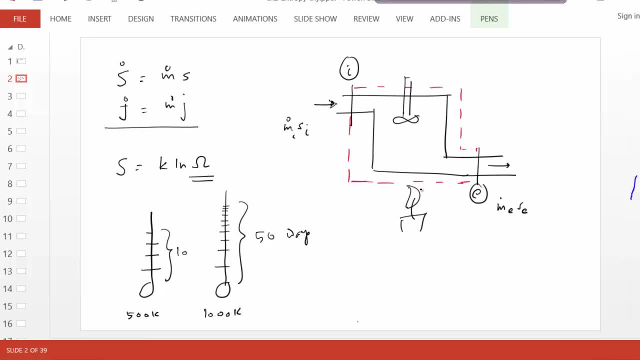 But in general there is always molecule to molecule transfer. So the molecules on the red boundary Is that Having higher kinetic energy than the molecule inside. As a result, these molecules, which are more energetic, are passing on energy into the molecules inside the systems. 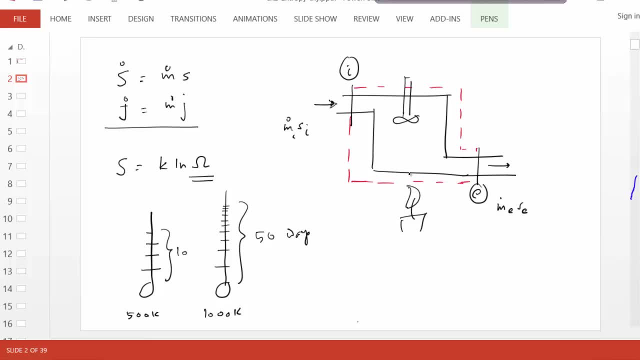 So, of course, if there is more, heat is transferred, as the molecule is passing energy from one molecule to another, And it also passes its own different energy levels. In other words, heat transfer always Carries entropy with it. What is even more difficult to understand is that the amount of entropy transfer is given by is proportional to heat transfer. 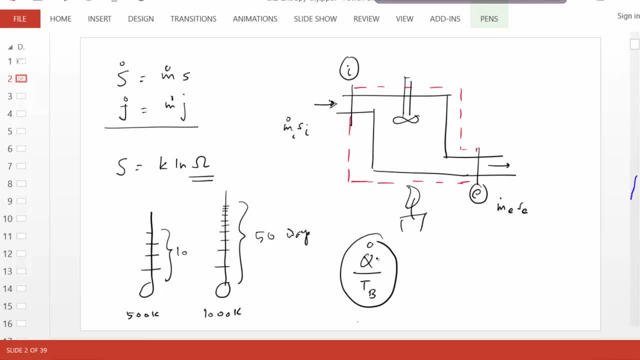 But it is moderated by the temperature of the boundary. In other words, if the boundary temperature is very high, the entropy transfer is a little bit less. Look at this relationship- inverse relationship. That's kind of a little bit difficult to understand. 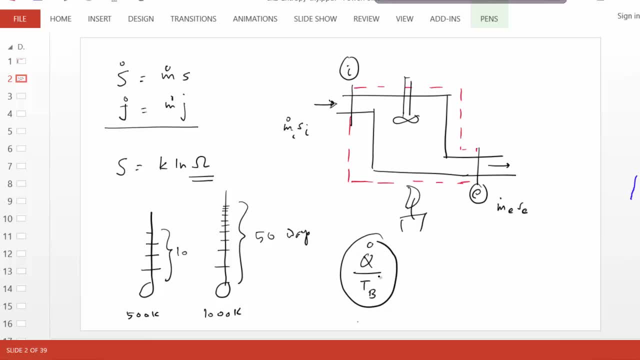 One will think that if the temperature is higher And molecules having more number of ways, How in the world the entropy transfer is decreasing in that case? Well, think about it. When the temperature is really, really high, Suppose this is the boundary molecules. 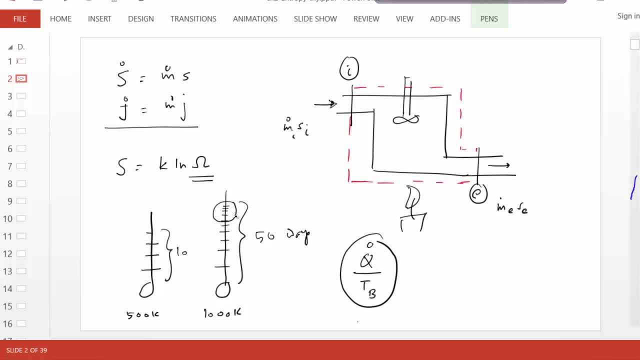 Then look at what happens. Most of the energy levels Are so concentrated These are not uniformly distributed. As temperature is higher, the higher energy levels are very close to each other, So most of the molecules at high temperature will probably be in this zone. 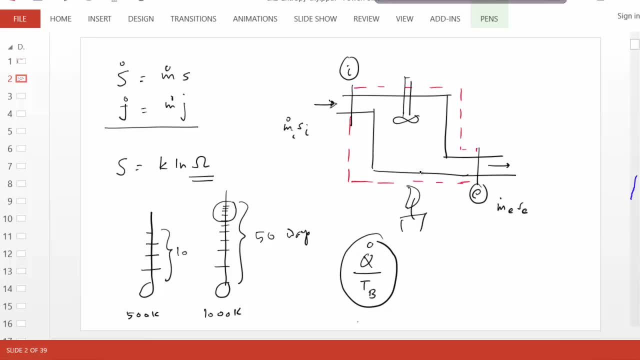 As a result, Because of entropy transfer, The energy levels we are talking about, They don't have so much variation, Whereas the boundary temperature is lower. Suppose the boundary temperature is 500 Kelvin, Then probably the molecules will be over a bigger range. 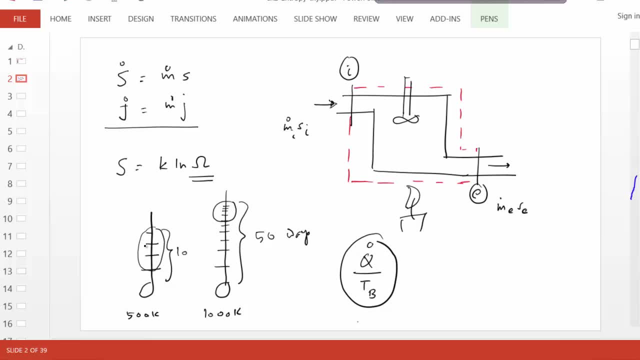 And, as a result, Because the energy levels are more sparse in this case. So, therefore, The variation introduced, The number of ways in which you can store things, The variation introduced will be higher At lower temperature. Well, it's more complicated than that. 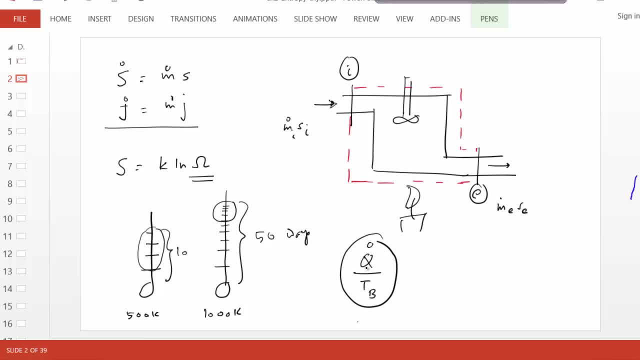 Derivation of this is quite complicated through quantum mechanics, But there are other ways in which you can get to that principle. But we will just axiomatically mention That whenever there is a heat transfer It carries entropy. So if heat enters the system, 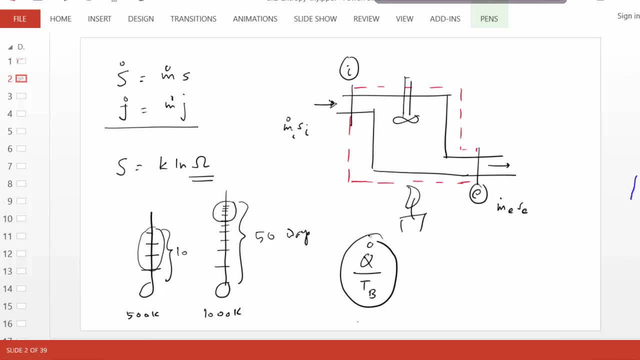 Not only energy has entered the system. There are more number of ways in which energy can be stored. As entered the system, Now there are more chairs in the room. Think like that, So there will be more ways in which energy can be stored. 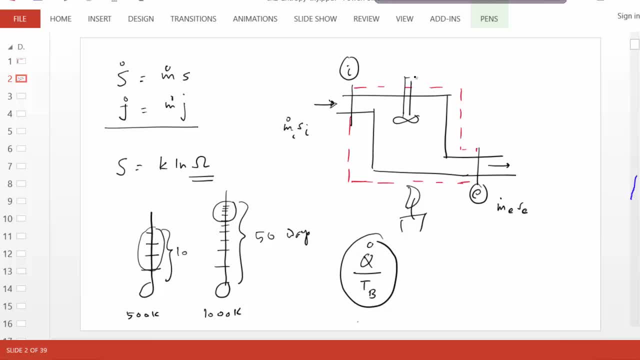 On the other hand, When work crosses boundary, Let's say, in this case, the shaft work, All the molecules of the shaft are moving the same way. There is no randomness, There is no levels associated with it. So, therefore, When external work, such as shaft work, 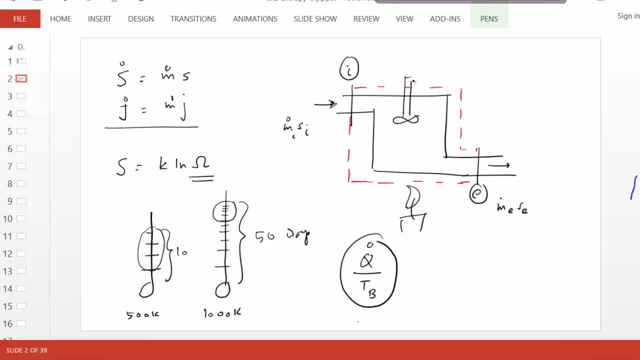 Electrical work Or boundary work crosses the boundary, There is no entropy transfer. So W dot external Does not carry Entropy. Why? Entropy is a measure of disorganization, As given by Ln omega Logarithm of the number of ways in which energy can be stored. 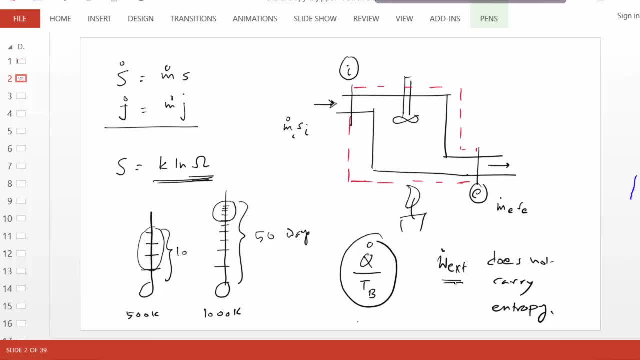 And External work Being All about organized energy. When a baseball- You know, Suppose Baseball- is moving at a constant speed, All the molecules are moving at that speed. These are organized kinetic Or kinetic energy. The Organized kinetic energy of the molecules. 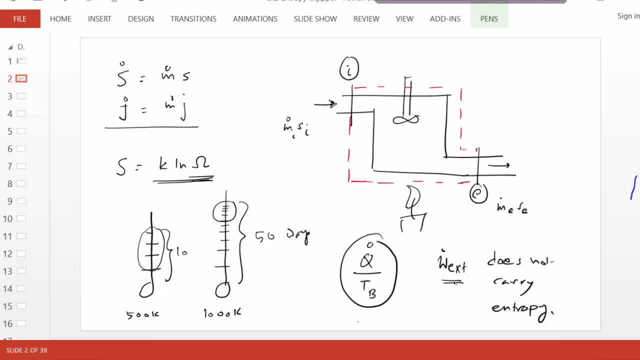 As opposed to U, Which is composed of the disorganized kinetic energy of molecules, Disorganized potential energy of molecules. So When there is external work, Say The shaft work, In which case All the molecules of the shaft moves the same way. 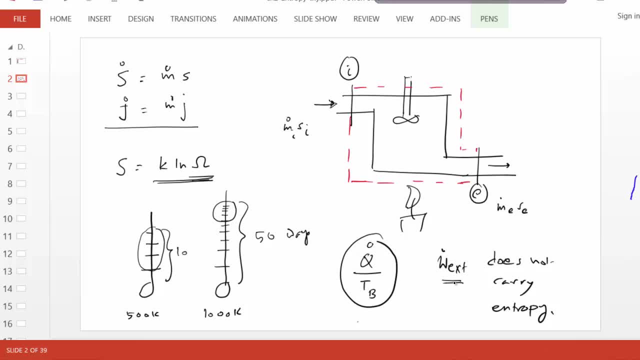 Electrical work, In which case All the electrons move the same way. Boundary work: Suppose a piston is moving down, All the molecules at the boundary are moving at the same way. There is no entropy transfer. On the other hand, During heat transfer, 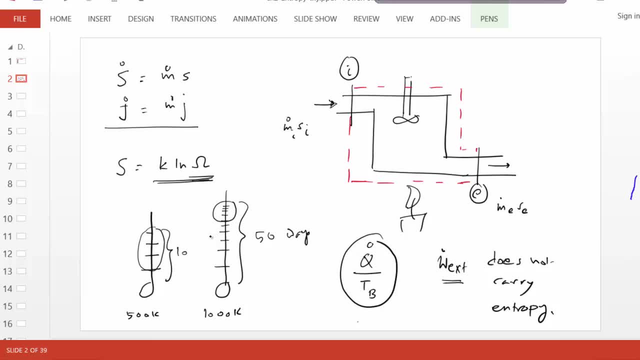 There is all this randomness involved. You don't know which energy level is going to be activated When some heat is transferred, So The hot gas. Suppose you touch A hot plate, Then the hot plate is not only going to transfer heat to your finger. 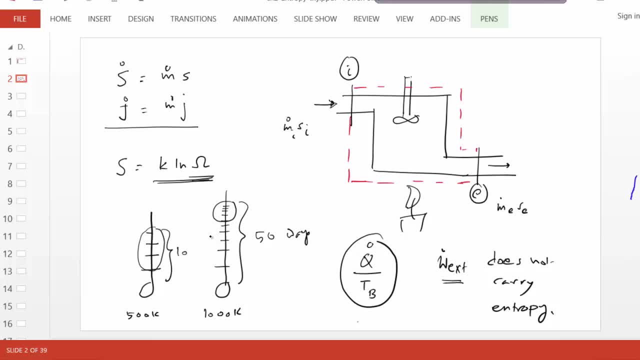 It is going to bombard your neurons here With different kind of energy levels. As a result, Your body Will get entropy from this hot surface. How? Because different energy levels are hitting your Molecules on your fingertip As a result. 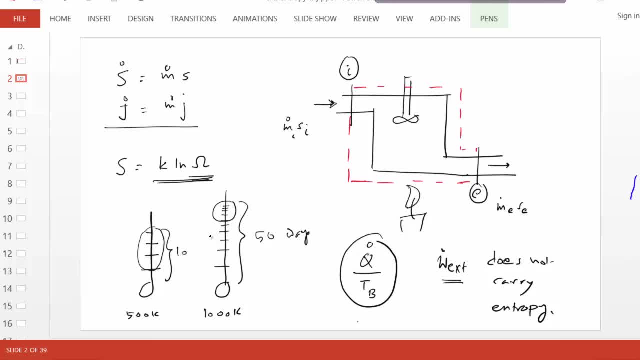 All these molecules Will be activated at different levels And Increasing the number of ways in which energy is stored, And So all you need to know in this case Is the boundary temperature: Temperature at which the heat is crossing the boundary. 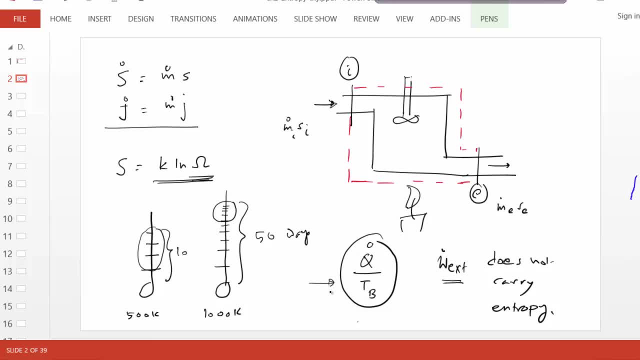 And this will be our measure of How much entropy is crossing the boundary. So, taking a look at this system again, Entropy can be coming in with mass. That's simple to understand. Any lump of fluid will carry Energy Entropy. 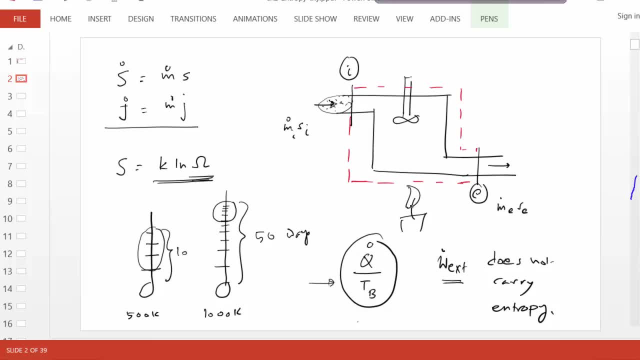 Kinetic energy. This is called transport. Entropy can also come in Because of heat And the amount will be Q dot By T B Per second, And no entropy crosses Because of External work. Now there is only one more way. 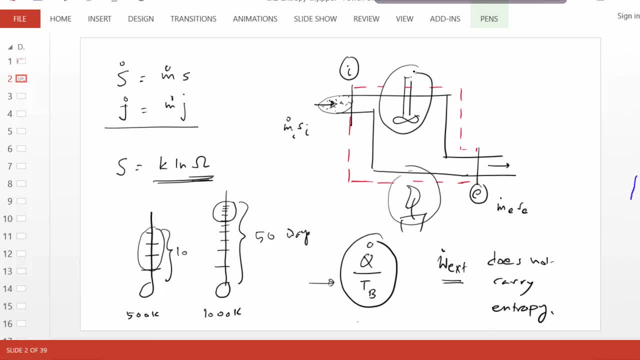 In which entropy Can be affected in a system, And that's quite important. The way in which Entropy can be affected Is called Entropy Because of heat, And the amount Will be Q dot By T. 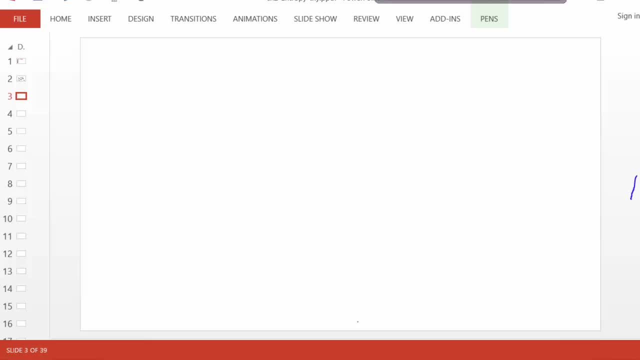 B Per second And no entropy Crosses, Because of External work In which Entropy Can be affected Is called Entropy Generation And that's quite important To Have a handle on And that's what is connected. 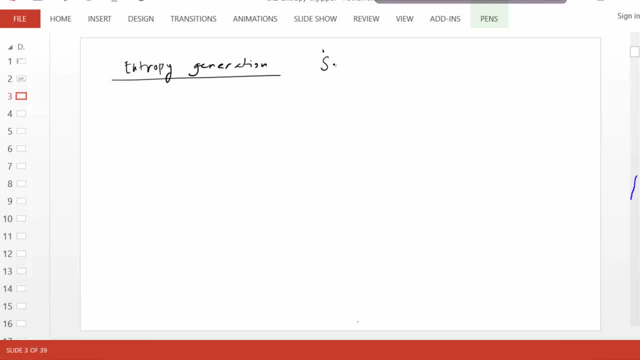 With the second law Of thermodynamics. So let's understand. What is The entropy Generation Rate S Dot Gen? Well, That's what makes Entropy So important, Because There are Natural Phenomenon. 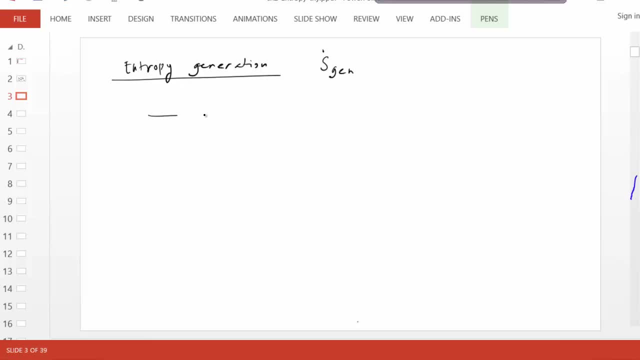 When, Where They Destroy It. I Give You A Simple Example. Suppose: Here Is Two Identical Block Of Metal. One Is At Thousand Kelvin And 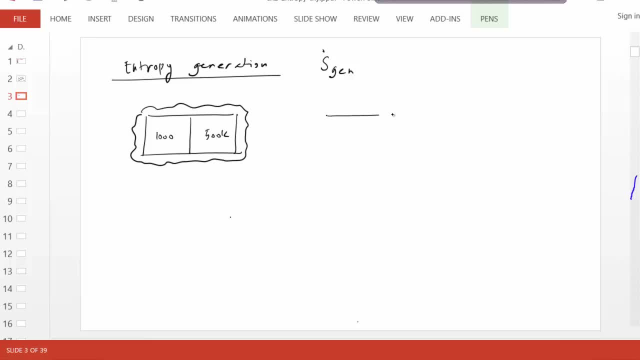 One Is At 500. Kelvin And Two Blocks Will The Temperature Equilibrate And Let's Say It Become Both, Become 750. Kelvin. We Know. 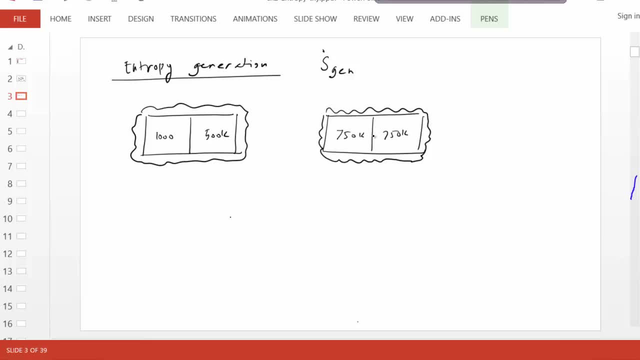 Fundamentally, This Is What Happens Even Without Any Idea Of Energy Equation. So If We Drop A Drop Of Ink In Clear Water, You 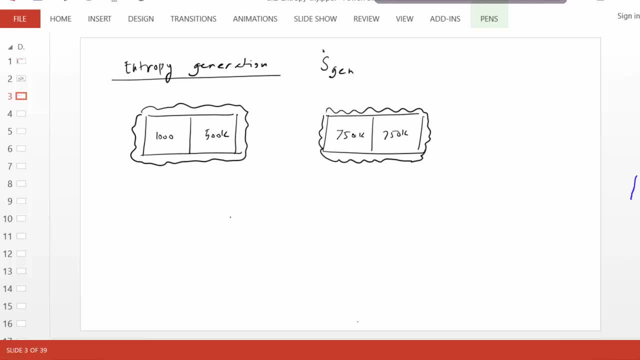 See The Concentration Difference Being Destroyed. If You For Instance Have A Voltage Difference, A Current Will Have Another Friction When Fluid Layer Passes. 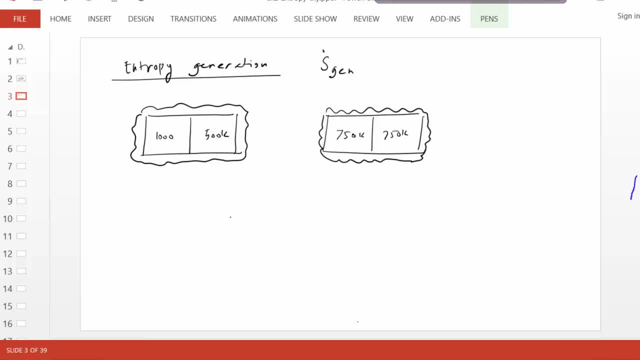 Over Another Fluid Layer, Viscous Friction Will Try To Stop The Motion. So In All These Cases, Natural Things Are Happening In The World. 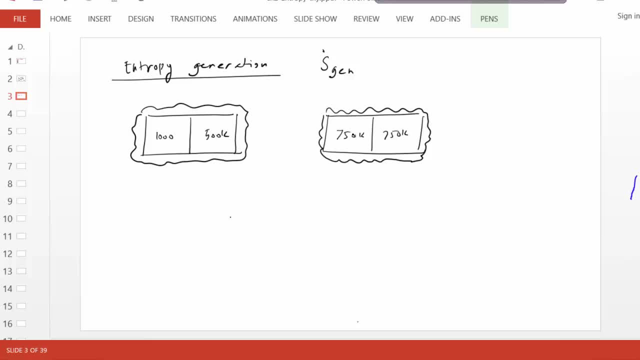 So We See That Signature Everywhere And The Second Law Of Thermodynamics Is All About It. If You Want To Say That In Language A, 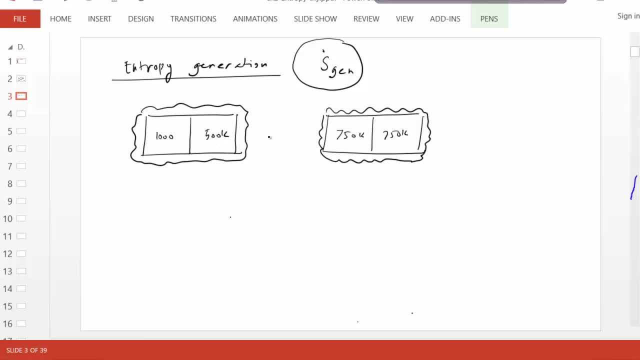 Second Law. To Simplify, Just To Illustrate, Suppose Only There Are Two Molecules, And So Therefore The Total Entropy Means What, In How Many? 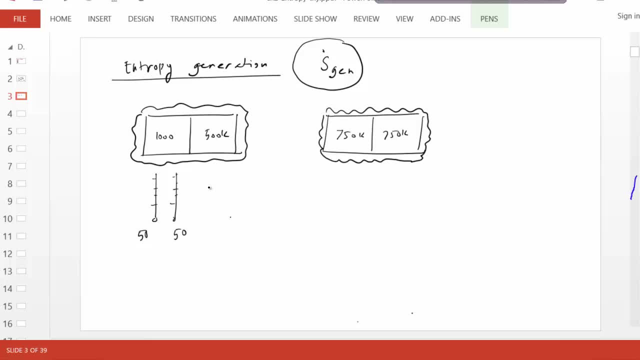 Ways Energy Can Be Stored, And This Is 10. Different Ways, So The Entropy Will Be Proportional To 50. Times 50. Times 10.. 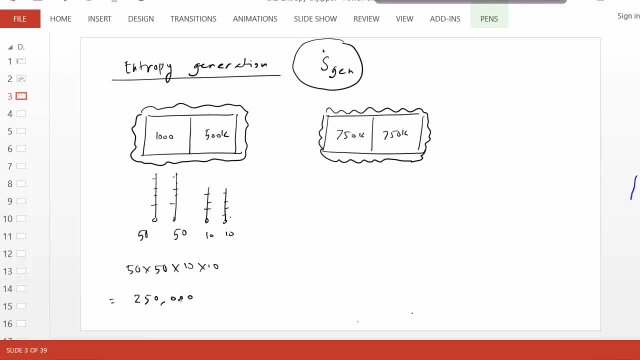 Times Tens Log Of That Anyway, But You Get The Idea Which Will Be Close And Each Molecule Now Will Have Less Number Of It. 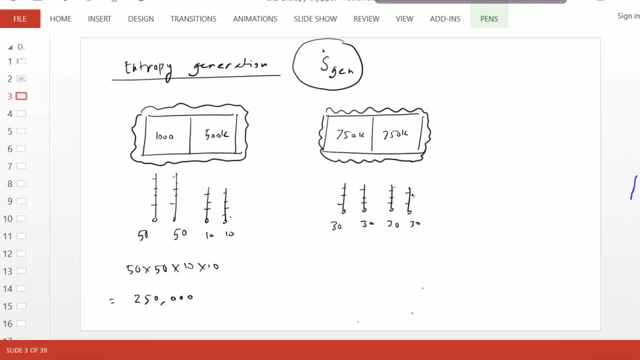 Will Be Somewhere Between 50. And 10. So Let's Say Somewhere 30. Ways In Which Energy Can Be Stored In This System And 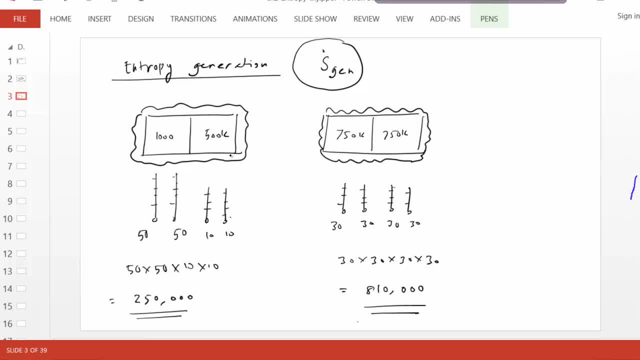 How Can It Happen? Entropy Is Not Coming Through Mass? Entropy Is Not Coming Through Heat. There Is No Heating. This Is Insulated, So 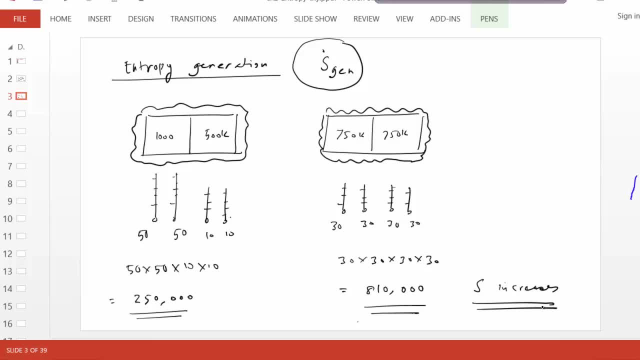 Entropy As A Matter Of Fact. It Can Be Shown That In All Gradient Destroying Phenomena, Entropy Increases. Entropy Is Generated Because 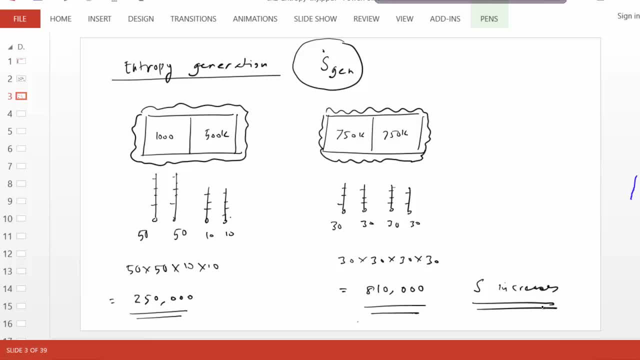 Of Entropy Increase If The System Is Closed, If There Is Not Coming Through Mass Entropy Is Not Shown In. All Matter Is Shown. 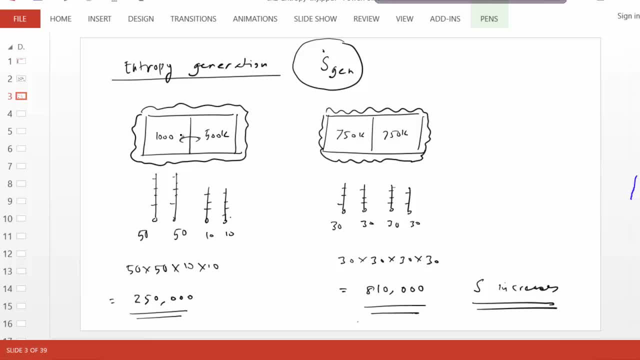 In All Matter. If There Is Entropy, Is Shown In All Matter Is Shown Is Shown In All Matter Is Shown Is Not. 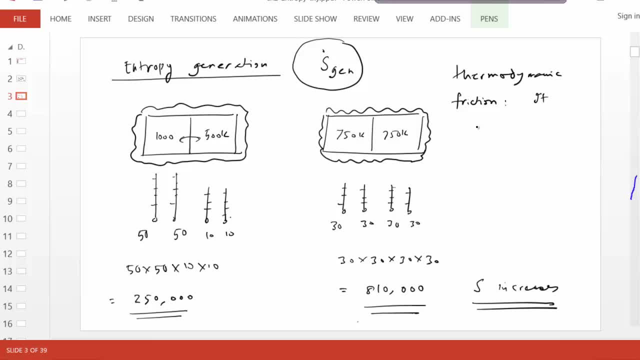 About That Triggering The Dibility Of All Matter Is, And A Resource Which Means One Killing The Other Thing To special change. So any difference in property when it's getting destroyed, we should immediately 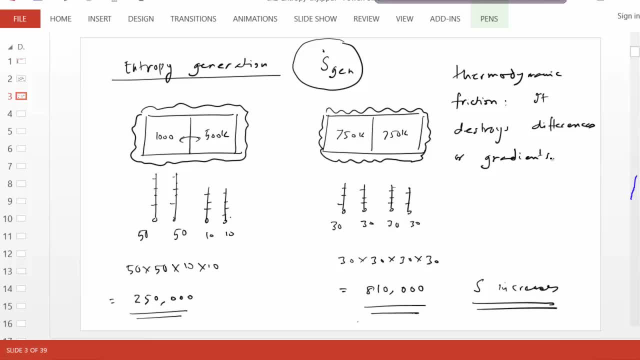 understand gosh, entropy will be generated So you can have an isolated system. suppose you have a cup of coffee, you stir it and you enclose it. you know the energy is not going to change because no energy is coming in or going out. but we know that the motion, if you start the coffee mug, the motion is: 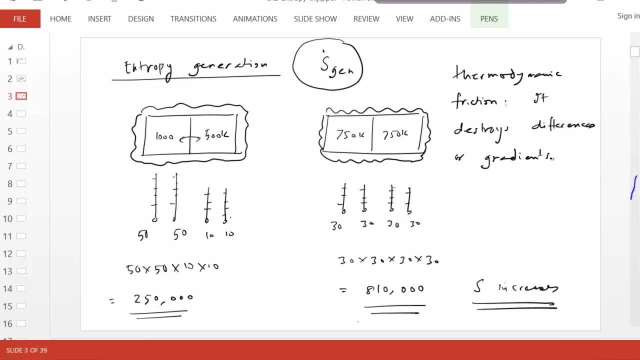 eventually coming to stop because of friction, and you can guarantee that even without going into each molecule and counting how many ways. you can bypass all this complexity by knowing that entropy will be generated, by immediately understanding entropy will be generated Exactly how much. for that we need the entropy balance equation. you can figure that out from: 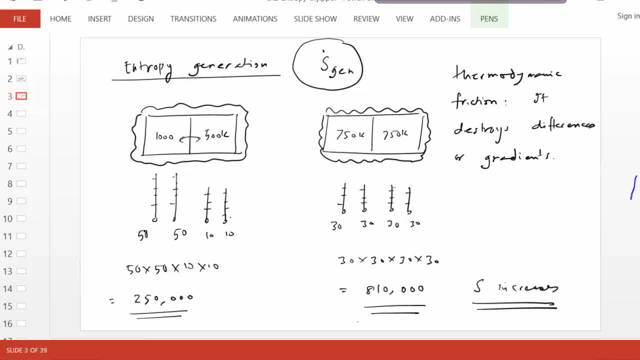 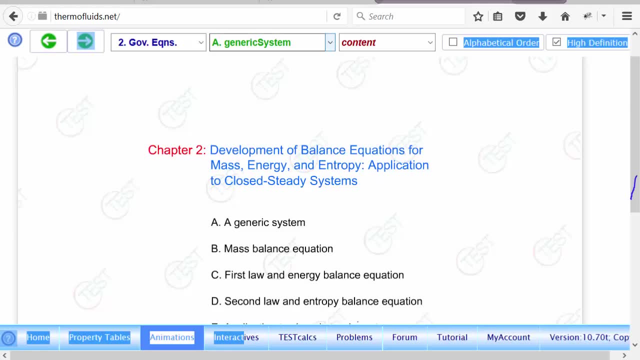 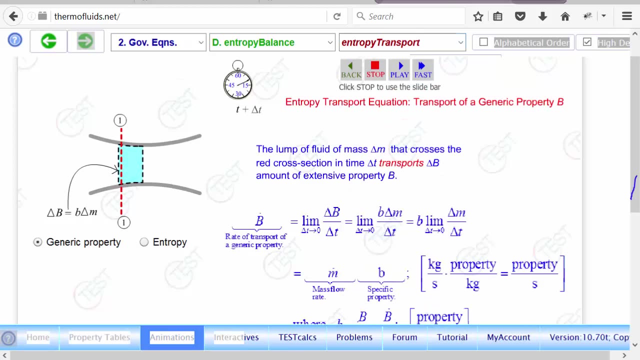 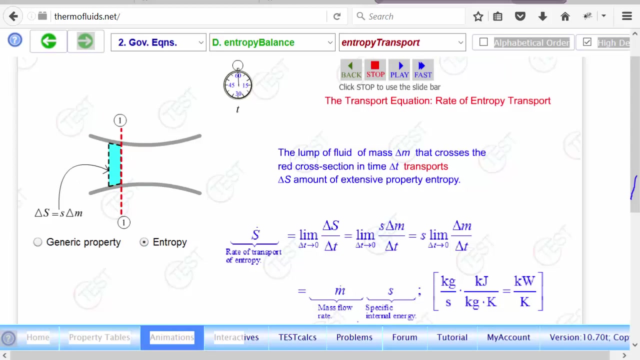 other terms of the equation. So to develop the entropy balance equation, let's go back to an animation Again. going back to chapter two, You go to the entropy balance equation again, just to just to remind you, this is the entropy entropy transport. we talked about m dot times s that a mass can carry entropy and we also 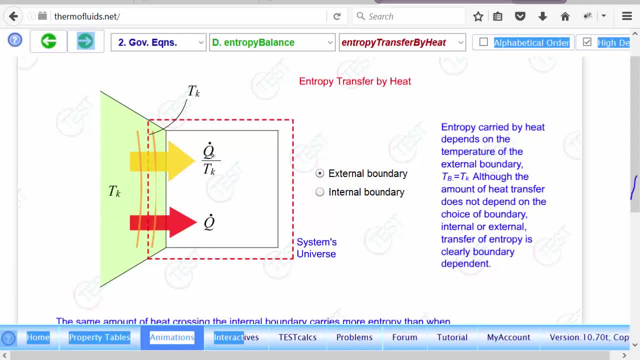 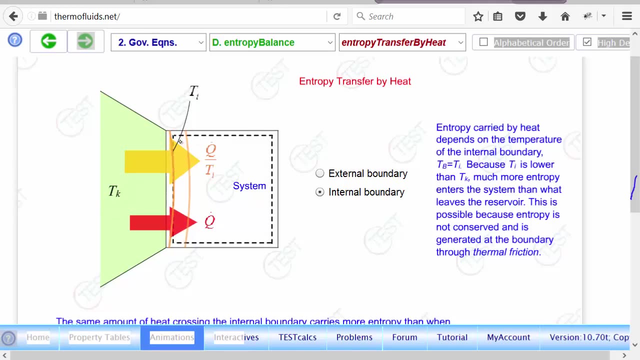 discussed how heat transfer can carry entropy q dot over t k. as you can see, the entropy transfer by heat depends on the boundary temperature. in this case the boundary temperature is TK. if the boundary is somebody picks a different boundary, it's called internal boundary. in that case Q dot- same heat is crossing the boundary. 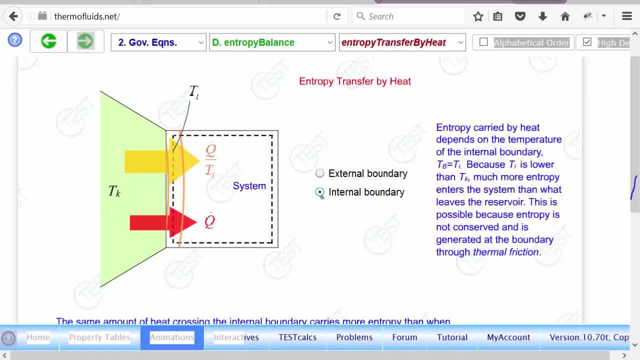 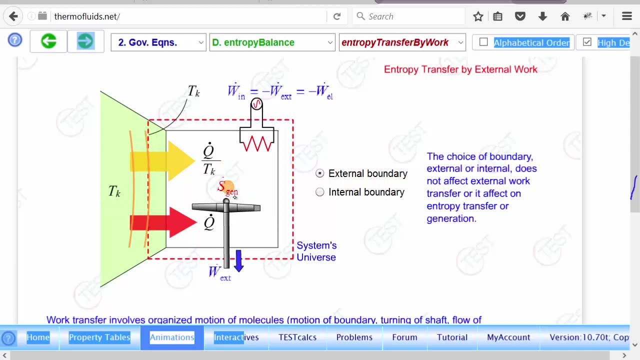 however, the temperature is different, so therefore, a different amount of heat will be crossing the boundary. entropy will be crossing the boundary. this is something that we'll explore later on again. finally, entropy can be generated, as they explain. in this case, the paddle wheel is causing a lot of friction, so 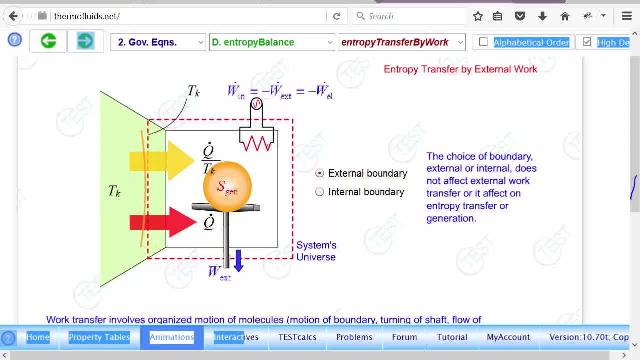 the question is suppose: what do you think about this resistance heater? electricity is crossing the boundary. we know electricity is not carrying any entropy. however, when the electric heater is getting hot, there'll be heat transferred. there is a voltage difference getting destroyed and there is a heat transfer from the coil to the, to the medium inside and therefore there. 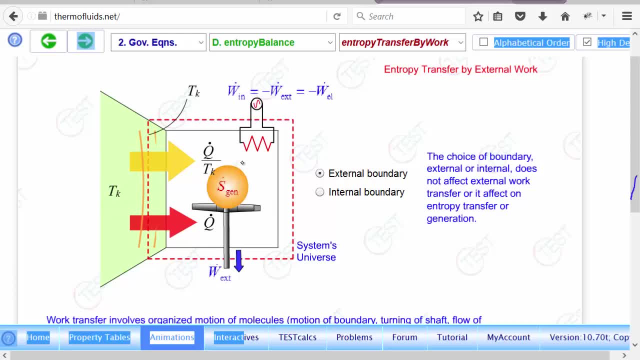 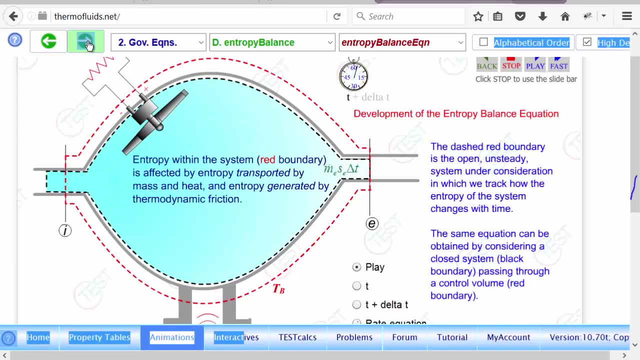 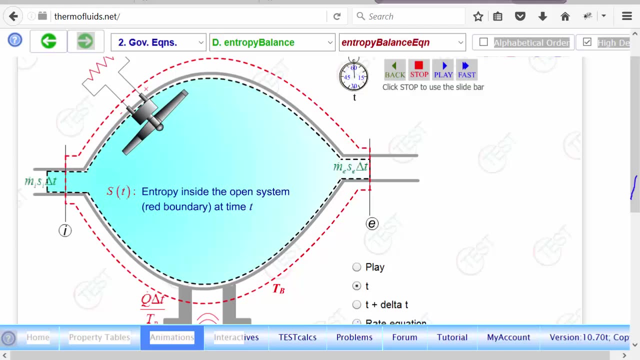 is thermal friction, electrical friction, so there is all kinds of reason for entropy to be generated. finally, to derive the entropy equation, now we have all the ingredients. at time T, we have certain amount of entropy within our red boundary, the boundary of the open system, and in time, 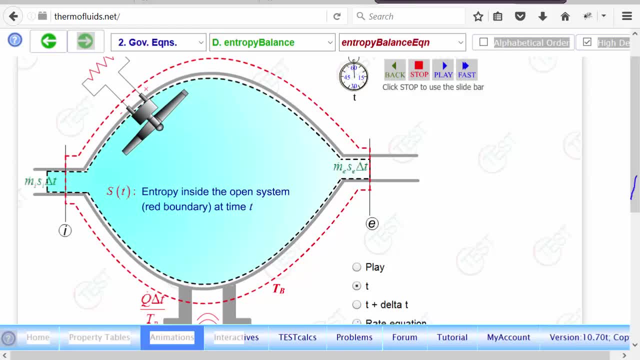 Delta T, we can see that entropy can come in through mass transfer. entropy can be transported out by mass transfer and the heat transfer divided by TV. this is the rate of entropy transfer times. Delta T: this is how much entropy is coming in through heat transfer and the work. 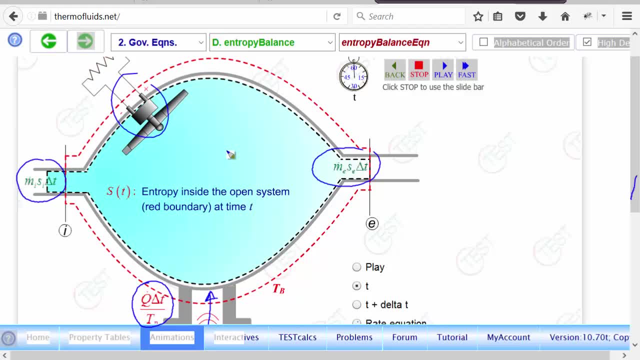 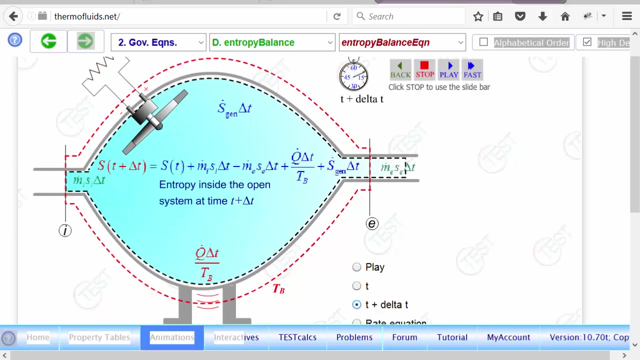 transfer doesn't have any impact of entropy. plus, there'll be entropy generation as dot gen times Delta T because of. we know, if there is friction inside the system, for a generic system, we must assume that there may be a thermodynamic friction. so at T plus Delta T, therefore we have the, the, the. 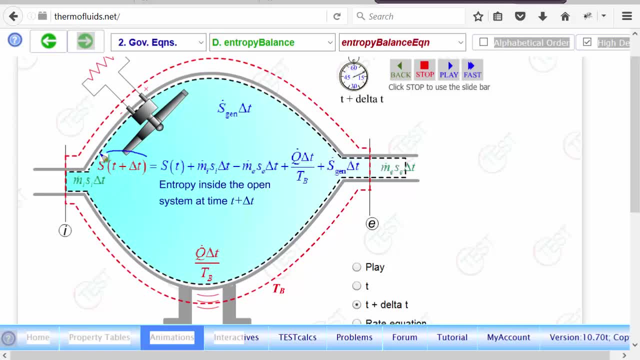 final entropy at time, T plus Delta T, is given by original entropy in the system: entropy that came in, entropy that got transported out, entropy that came in through heat transfer and the entropy that is generated because of friction within the system. so now that we have the complete inventory, 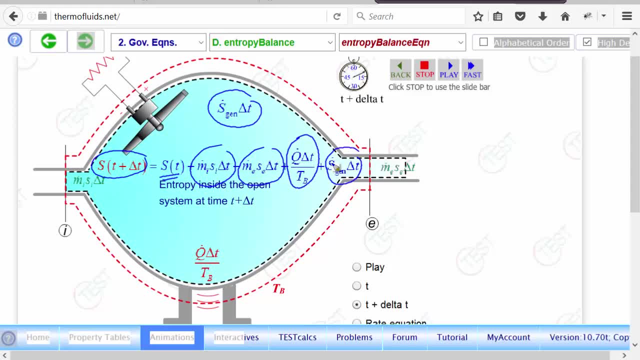 we also recognize that entropy can only be generated because of friction. there is no negative friction in nature. if there is, if there's a, you know, if your room is at 30 degree Celsius, you cannot suddenly come and find that the one side of the room became hotter, another side became colder. that will consider that will be. 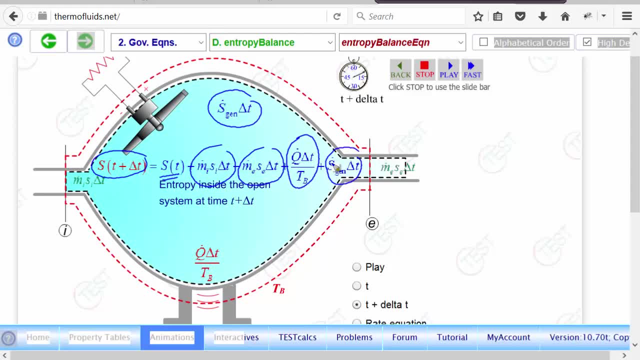 considered negative thermodynamic friction. so therefore, at s dot gen, entropy generation can never be negative, and that's the second law. second law means entropy generation rate can be 0 at the best, or positive. friction can be absent in an ideal case, but friction can never be negative. that's what second law. 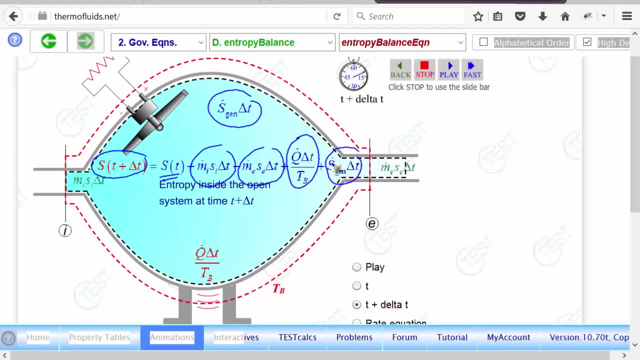 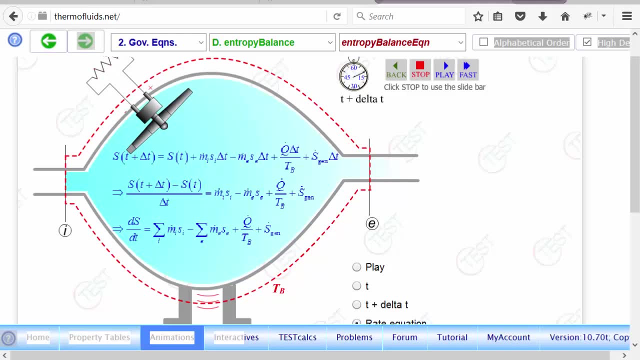 means, but the entropy balance equation therefore reduces to. if I go to the rate equation, we do the same thing we did for the mass and energy equation: change the sides divided by delta T, take the limit and what we get is the final entropy balance equation, which states that the rate of change of entropy of a 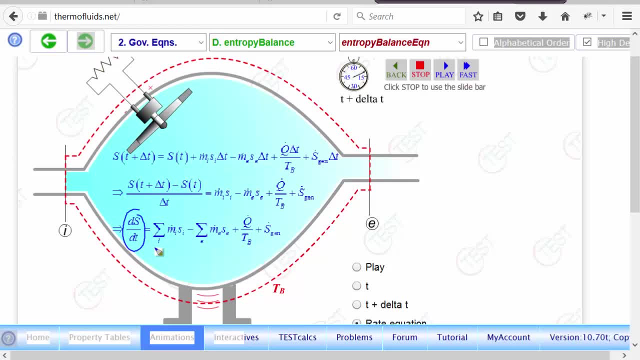 system. the unsteady term of the entropy balance equation is given by the transport terms: the entropy that is coming in here going out, minus what is going out there, summed over all the inlets and exits. entropy that is transferred by heat. we know always heat will carry entropy based on the boundary. 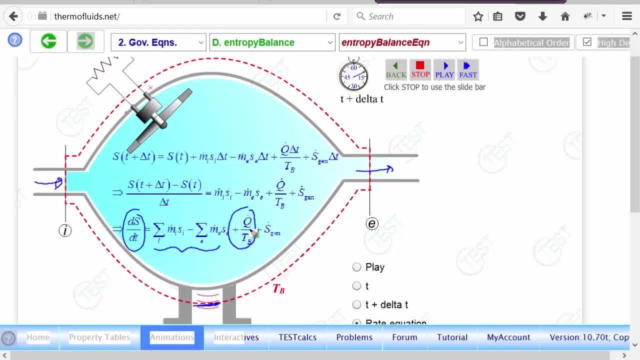 temperature. here T B is the boundary temperature, obviously, even though we show just one term, if there are more than different heat transfer, different reservoirs of heat, then we have to. we have to split that up into different terms: Q dot 1 by T 1 plus Q dot 2 by T 2 plus Q dot K by TK, like that, instead of complicating with. 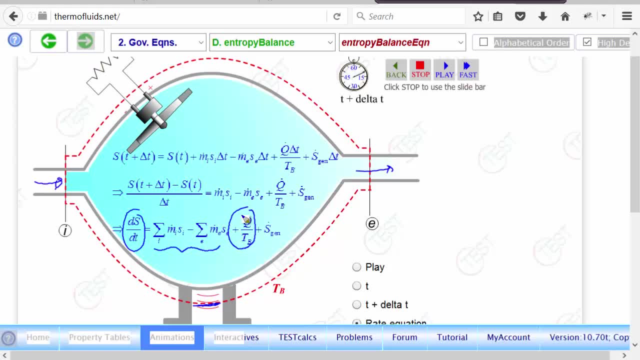 the summation sign. we are just showing it by a single term. and finally, entropy, generation term. that is the term that must be greater than equal to 0, which means entropy can be. there can be friction within the system and a lot of the time our goal would be to find that friction. we can do that by finding the 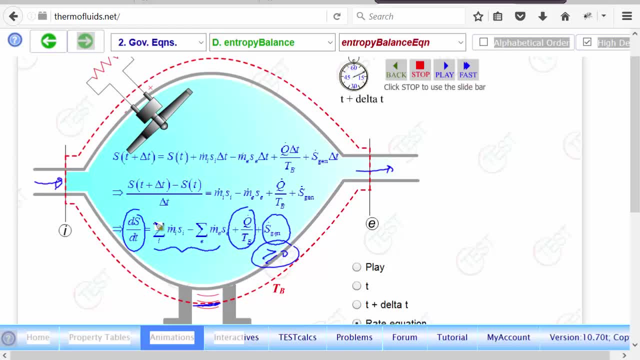 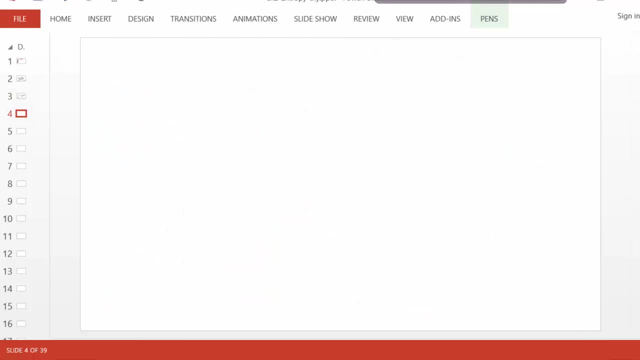 other terms in the equation and using the rate equation. so we'll solve a number of problems: who is using this equation and the meaning of this equation will become clearer as we solve more problems. so to summarize the rate equation for entropy, we can write: the DS DT equals sum of M dot I, SI minus sum of M dot E, SC plus Q. 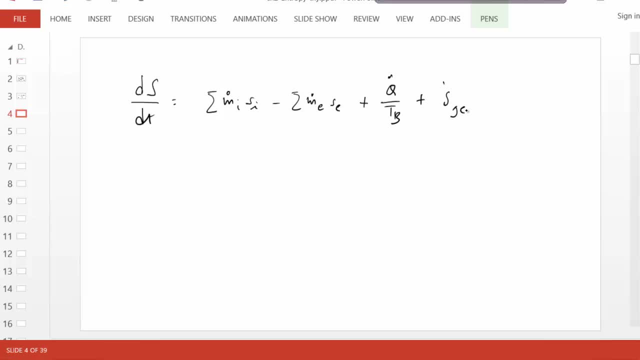 dot over TB plus s dot Chen. notice the unit for entropy becomes clear now. Q dot is kilowatt, TB is Kelvin, so each term must have the same same unit. so therefore you can figure out the entrop unit for instance. so M dot must be kg. 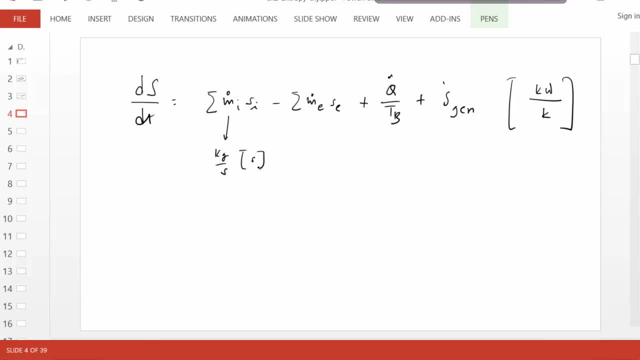 per second. so what becomes of the unit of entropy? together must be kilowatt per Kelvin so that you need of entropy. specific entropy must be kilowatt per Kelvin. second kg kilowatt is kilojoules per kg. sorry, kilojoules per second. second gets canceled, so you get kilojoules per kgk. 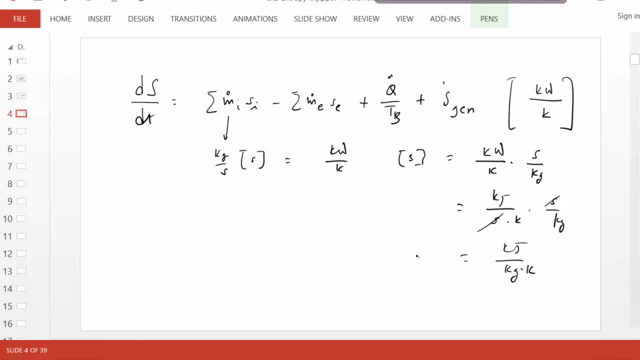 so that's that you need of specific entropy this week entropies. entropy per unit mass: as you can see, it's kilojoules per kg K and the unit of entropy capital K S, is kilojoule per Kelvin. So the rate of change of entropy of a system is given by the rate at